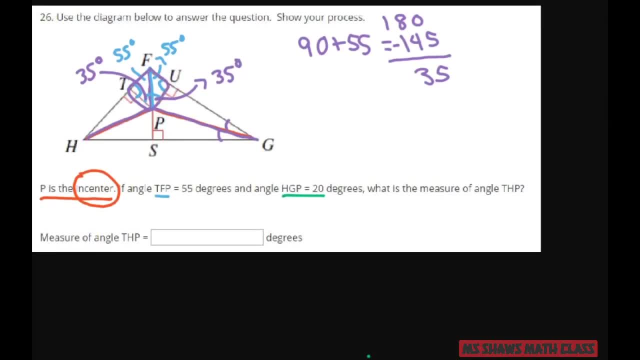 Now for HGP. So this triangle here, This angle is 20.. So this is 20.. That means this angle here It's going to be 70.. Because that gives you 90. And this whole triangle here will add up to 180. 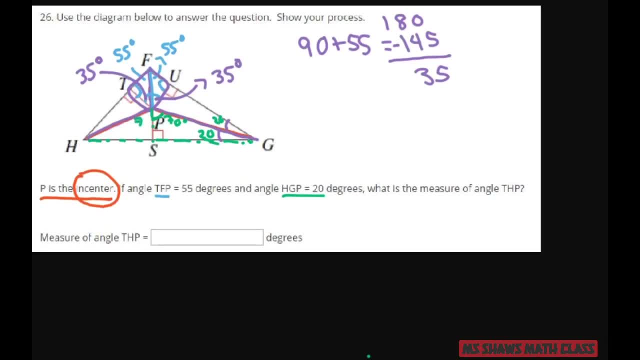 And that means, because it's a bisector, this side is also going to be 70.. Now let's look at what we have, And I'm going to draw a circle, And a circle has 360 degrees, So what we have. 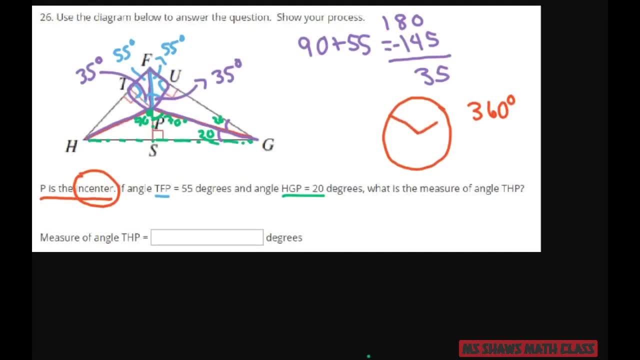 Is, we have this portion Here Which was 35 degrees And 35 degrees, And then we have this portion here. Let's see, Let me try to make something here. Alright, These two were 70 and 70 degrees. 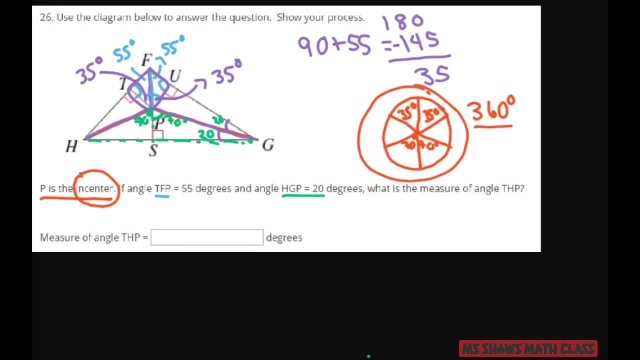 So all of this has to add up to 360.. But since we're talking about angle bisectors, That means these two sides have to equal each other. So these two- That's your end center- These two have to equal. 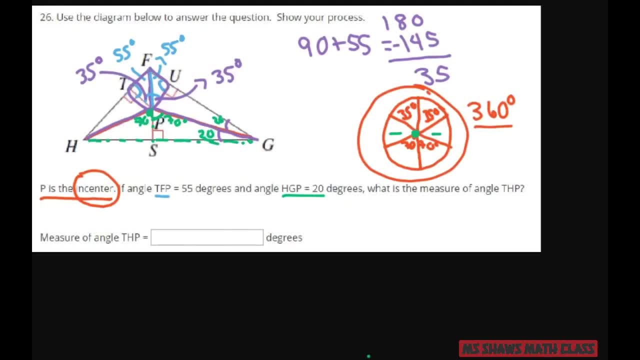 So if I add this up, I'm going to get 360 minus 35 minus 35 minus 70 minus 70.. Basically, It's going to be 360 minus 210.. Which gives you 150.. So if you take half of 150. 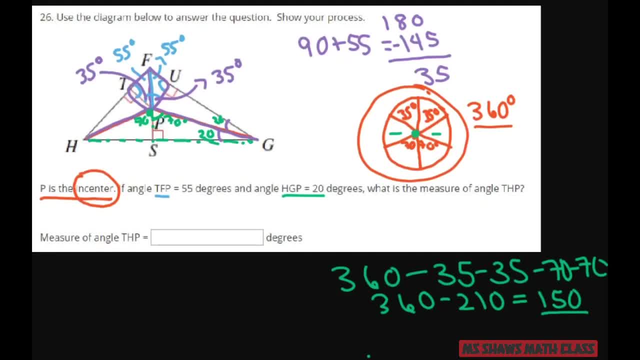 You get 75.. So this will be 75.. And this one will be 75.. So all these angles In this area- I'm going to kind of erase this now- In this circle area Should equal 360. 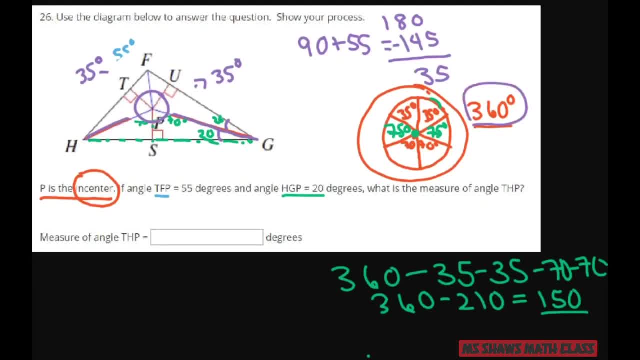 So for what we want, We want this part. So I know this angle. here is 75. So if you take 90 plus 75.. 90 plus 75 gives you 165.. And you subtract that from 180..